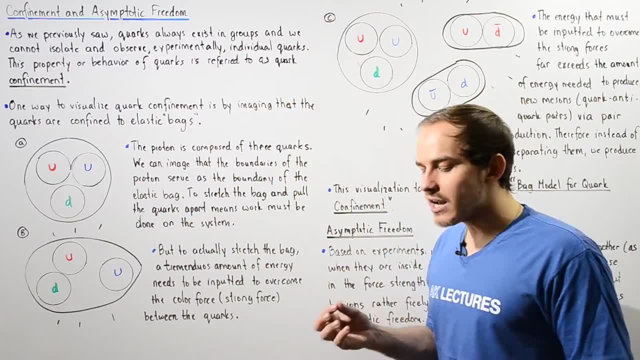 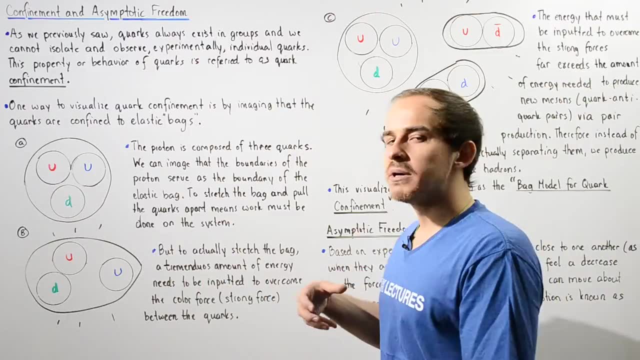 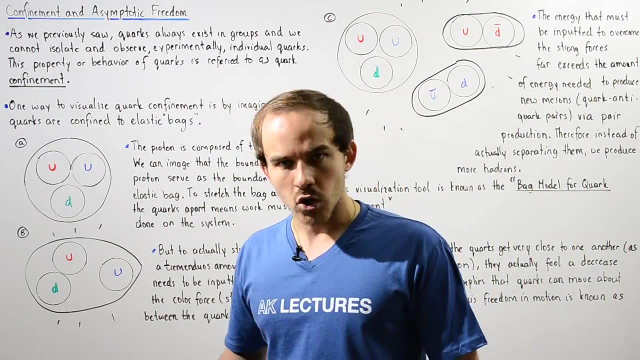 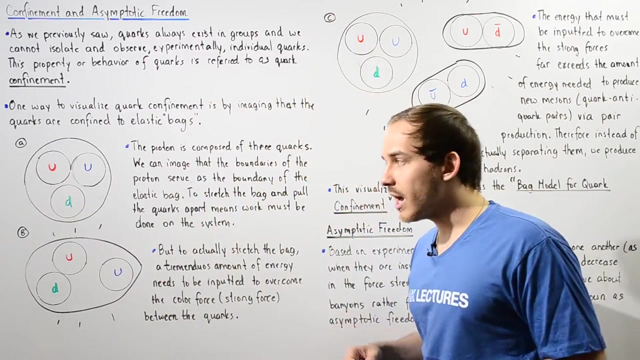 quark confinement is by imagining that our quarks are confined to an elastic bag, An elastic bag that can be stretched. But to stretch this bag we actually have to input a great amount of energy, a great amount of work. So let's take a look at diagram A. In diagram A we have one type of baryon, the proton. 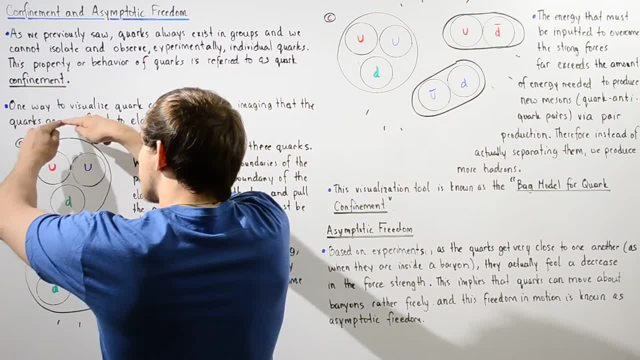 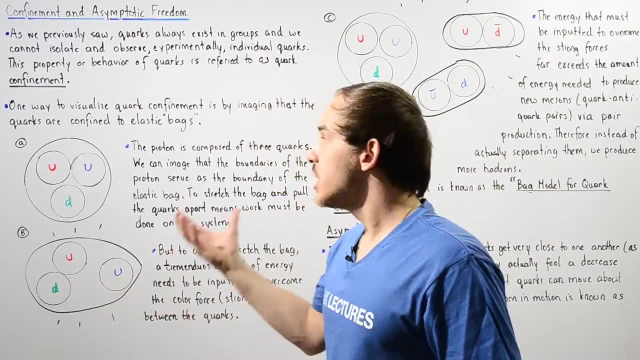 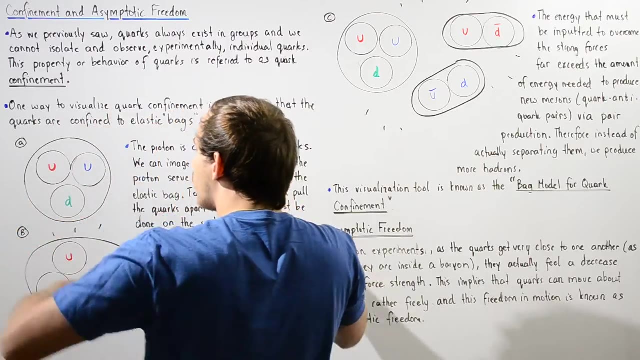 So the proton is shown by this outer circle And we can imagine that the outer boundary of our proton serves as this elastic bag. And to actually stretch the elastic bag to separate the individual quarks, we have to input a certain amount of work into our system. 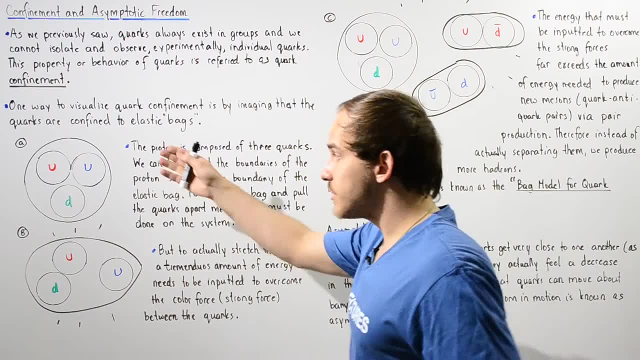 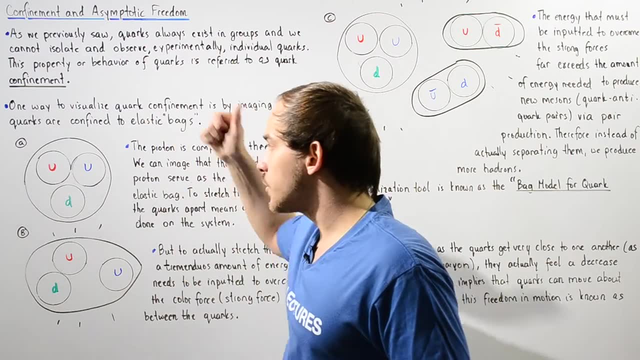 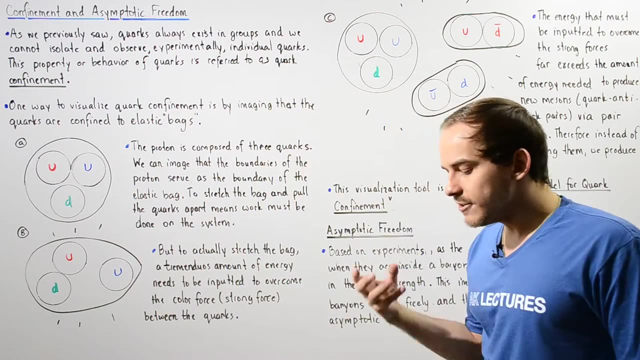 our proton. So basically, inside this proton we have three quarks. So we have the up quark, which has the color red, We have the other up quark that has the color blue, And we have down quark, which has the color green, And each one of these colors produces a color charge. It 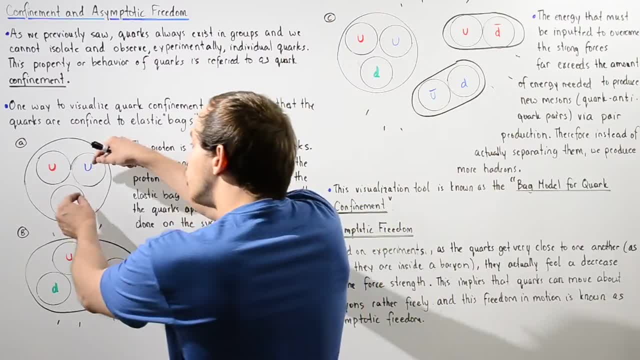 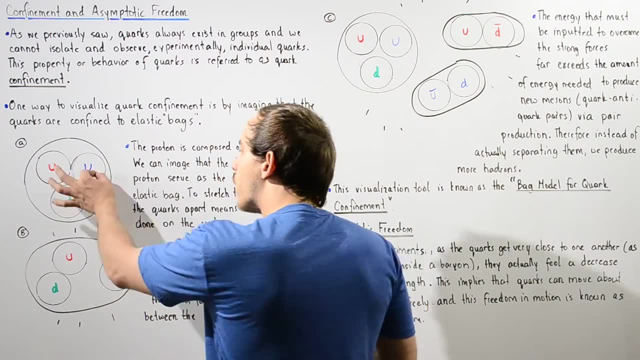 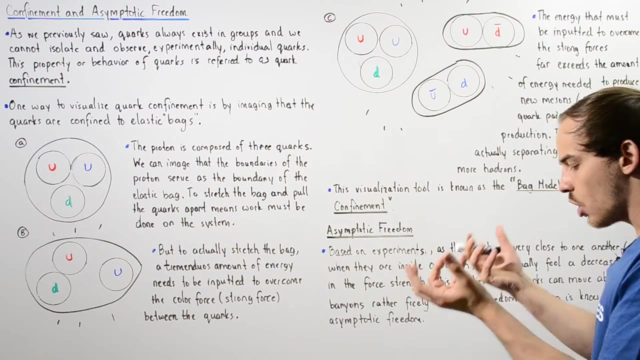 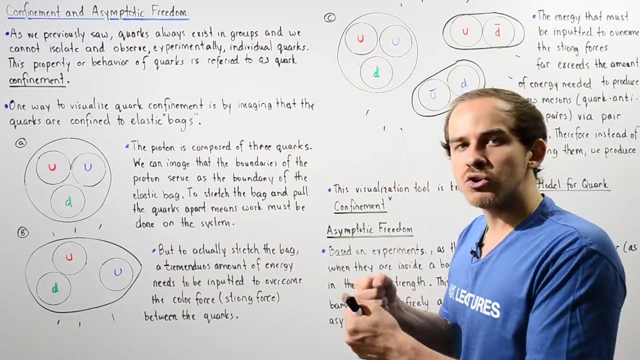 gives the quarks color charge And when the gluons, the fundamental particles that carry the strong force, also known as the color force, when they exchange the gluons. that basically holds our quarks together within our proton. Now let's actually suppose we try to separate our quarks. 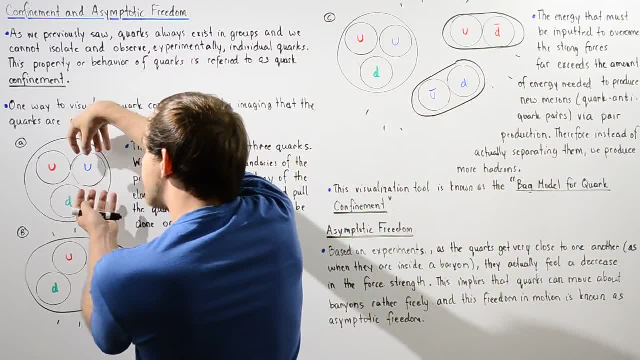 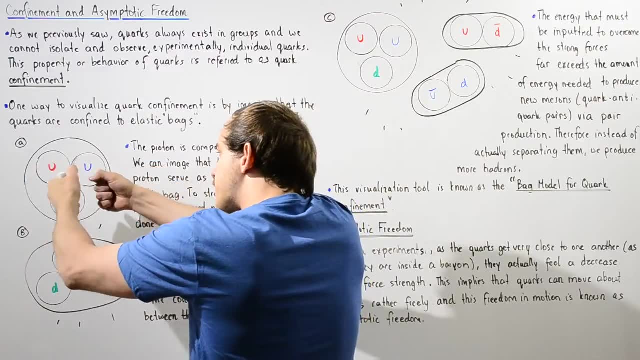 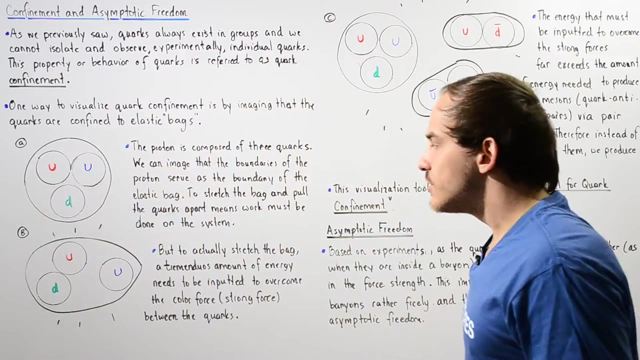 from one another. Let's say we want to separate this blue up quark from these other two quarks So we try to actually input a certain amount of energy, We try to do work on our system to separate our quarks So it actually turns out. 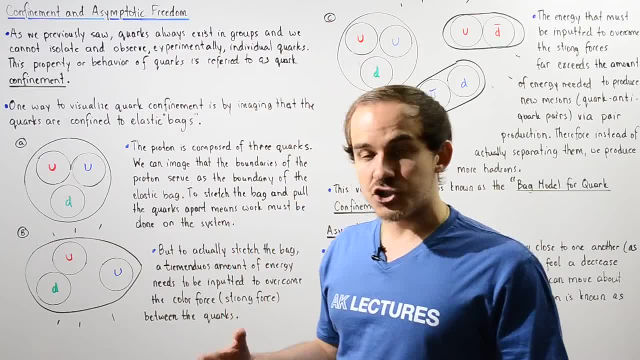 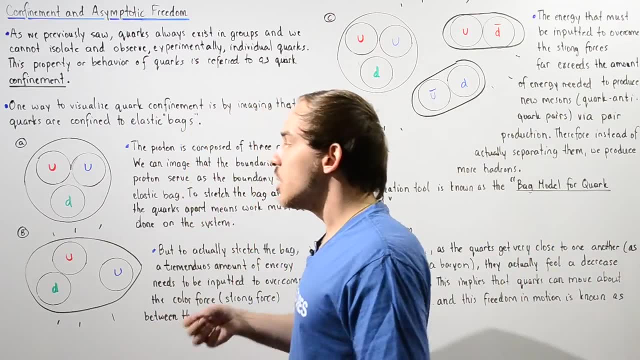 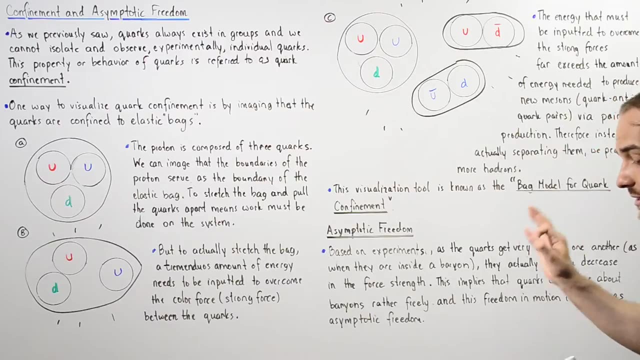 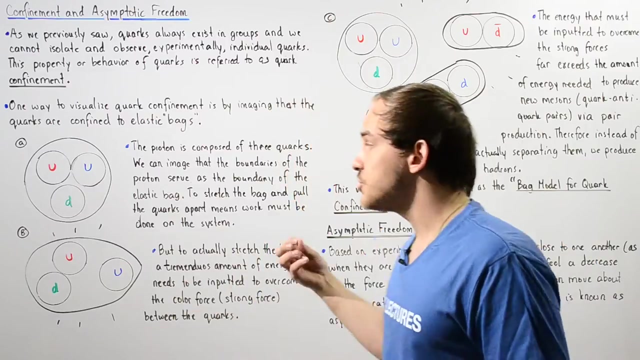 that a tremendous amount of energy, of work must be done to actually overcome those strong nuclear forces, those color forces that hold our quarks together. Now it turns out that when we actually input that tremendous amount of energy, the amount of energy that we input to actually separate, 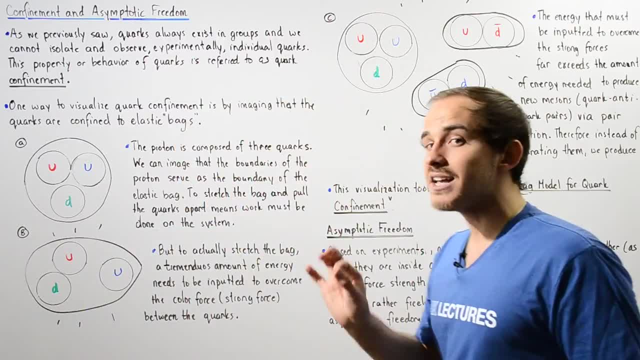 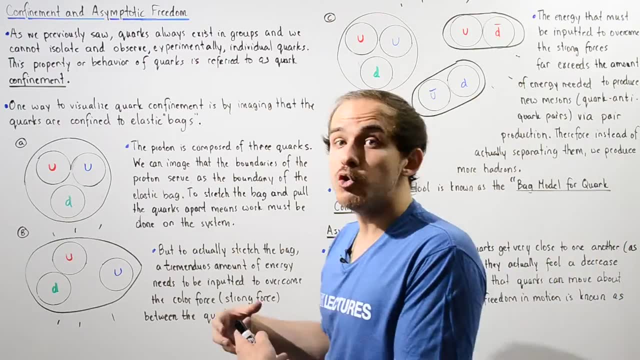 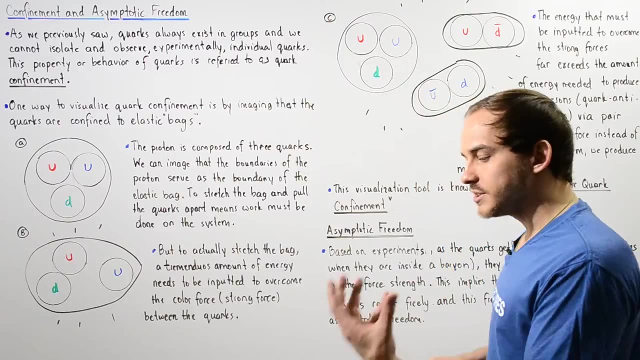 and stretch our elastic bag, that tremendous amount of energy that we put into our system ends up exceeding the amount of energy that is needed to actually form new mesons and baryons via the process of pair production. So remember, pair production is basically using energy to 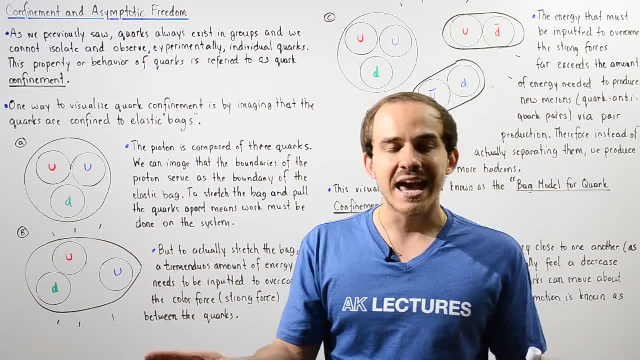 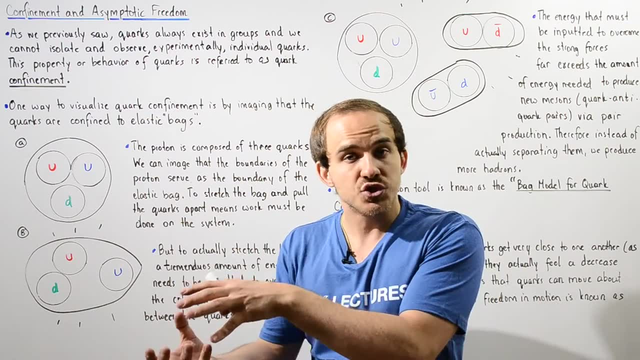 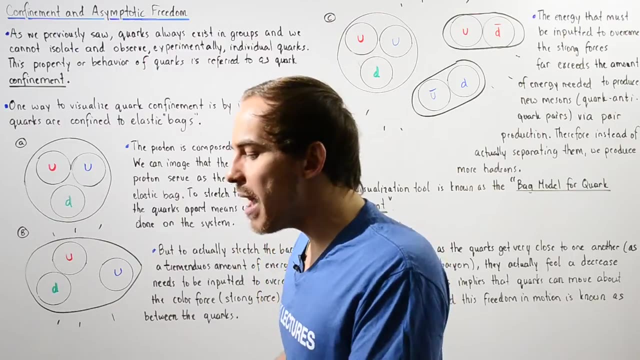 transform energy via Einstein's mass-energy equivalence principle, converting energy into mass. So recall that we can actually use energy and if we have a mass-energy equivalence principle and we have a great amount of energy, we can readily transform that energy into forming new mass. 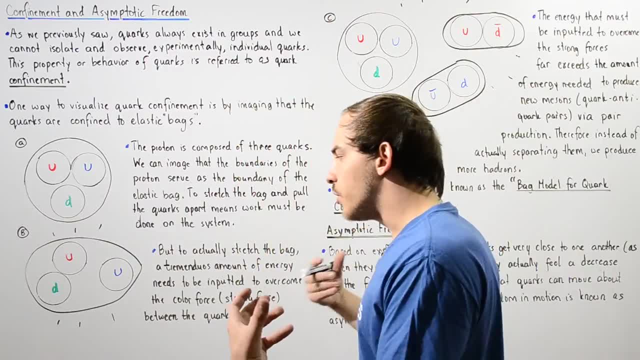 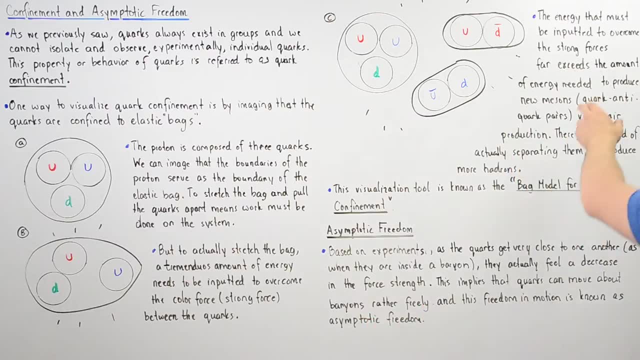 new particles, And it turns out, when we input this great amount of energy, we input an amount of energy that exceeds the amount of energy needed to produce new mesons- the quark-anti-quark pairs- via pair production, And this means, instead of actually separating, 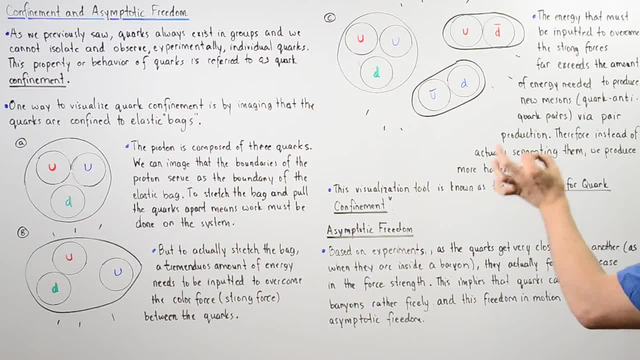 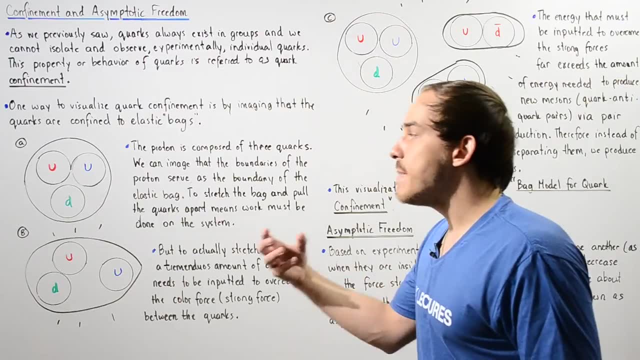 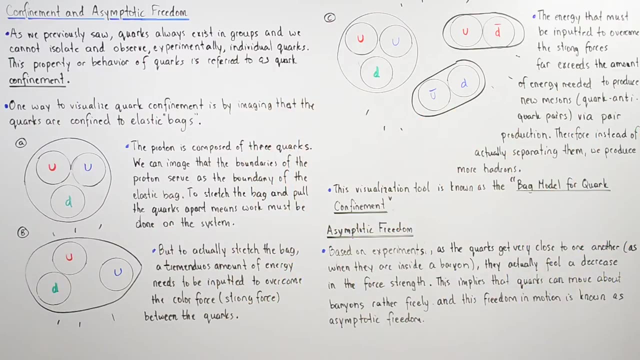 our quarks, we end up producing more mesons and more baryons, so we produce more hadrons. So this method of visualizing quark confinement is commonly known as the bag model for quark confinement. So one other concept idea that I want to discuss in this lecture briefly. 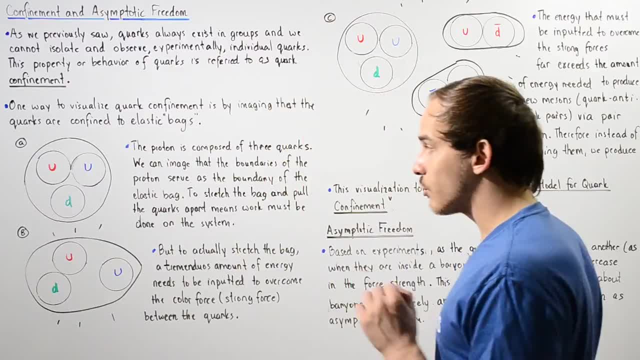 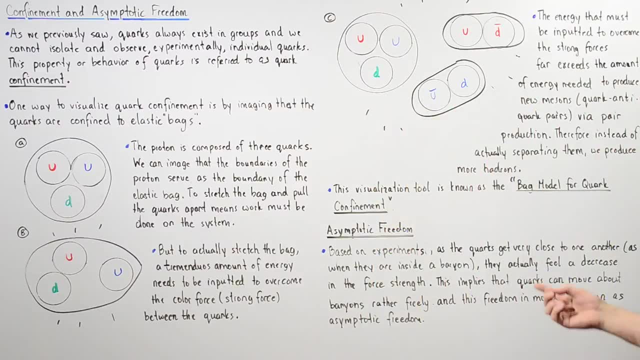 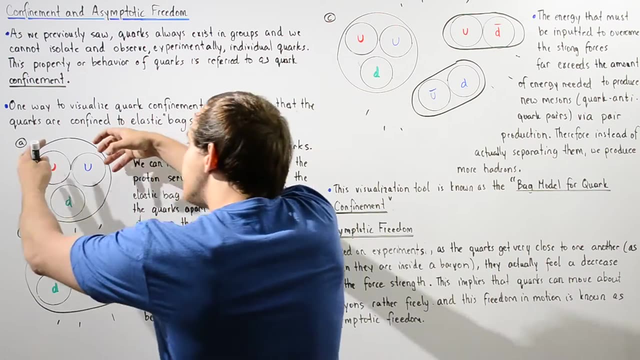 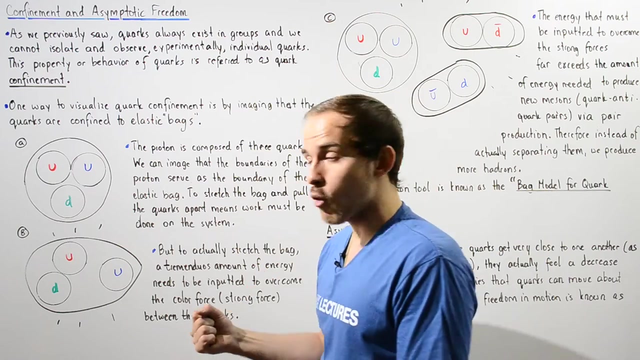 is known as asymptotic freedom of our quarks. So, based on experimental evidence and experimental results, we see that as the quarks actually get very, very, very close to one another, so when they get close enough to form our proton, we see that the color force or the strong nuclear force that exists between 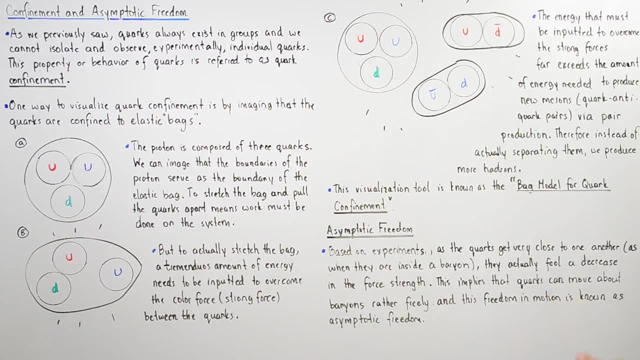 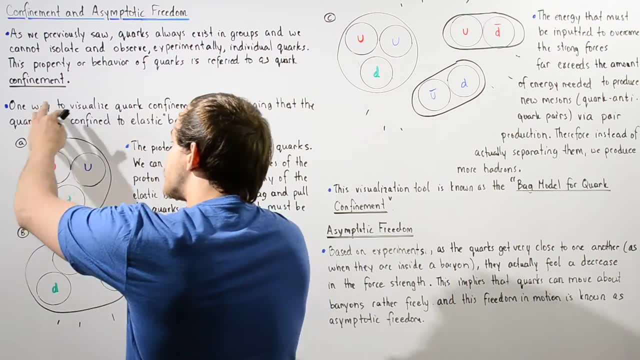 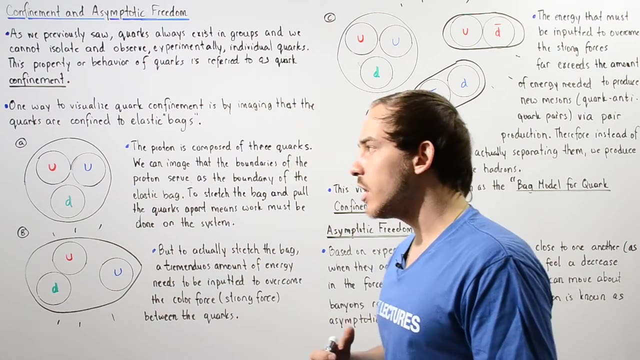 these quarks actually ends up decreasing And they can actually now move. uh, when they move with a great amount of freedom around the space of the proton. And this idea that as the quarks get extremely close to one another, the force decreases between those quarks is 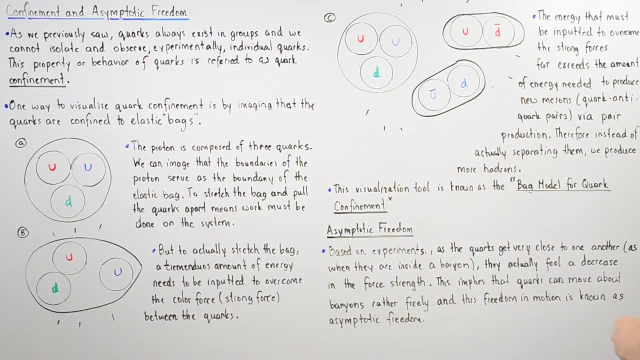 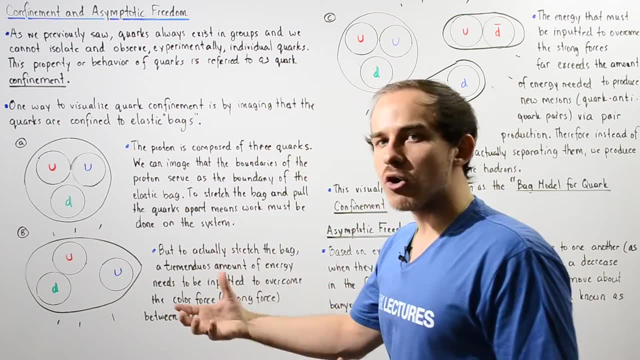 known as the asymptotic freedom of those quarks. Now, of course, as the quarks begin moving away, that force begins to increase once again. So this idea of our quarks actually being able to move to a higher bestimmtcy of mass and